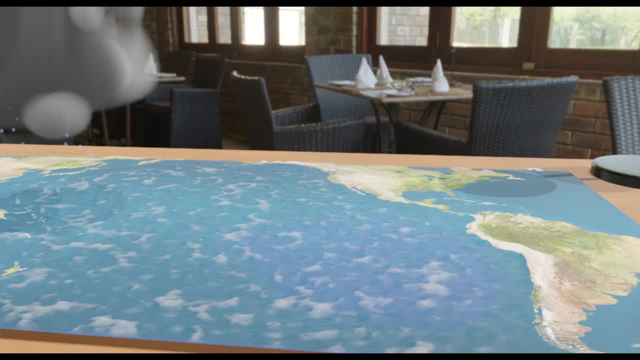 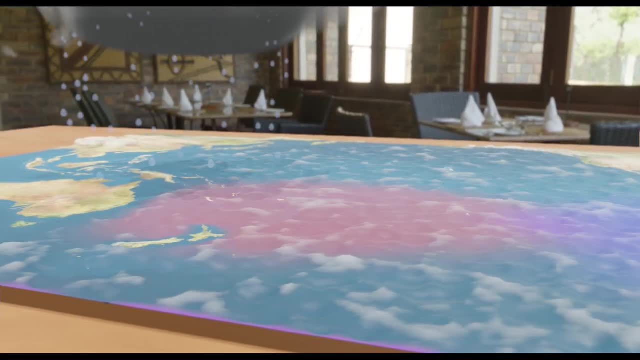 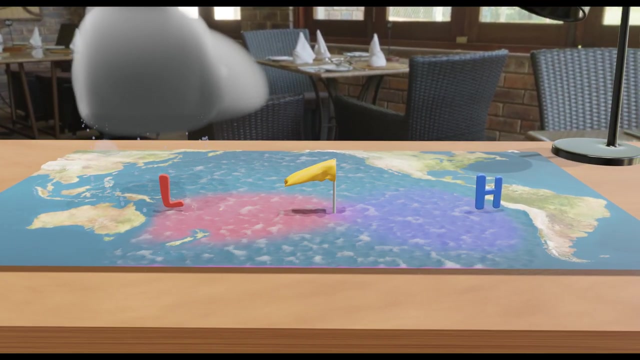 Pacific Ocean normally behaves. We have colder water over here, which cools the air and thus increases the atmospheric pressure. We have warmer water over here, which warms the air and creates low atmospheric pressure. As one would expect, the air flows from high to low pressure Normally. there should. 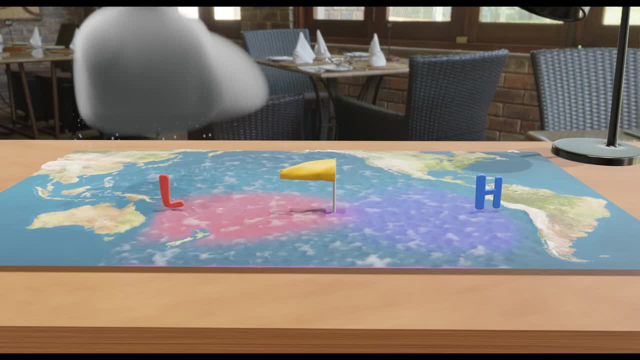 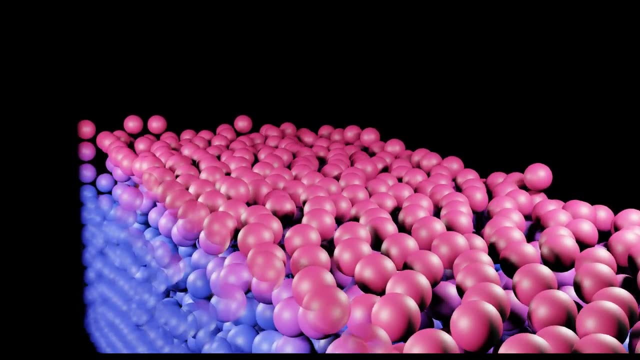 be no reason for this temperature imbalance, but since the thermocline is important, that probably has an impact. The wind caused by this difference in pressure tugs on the ocean via friction, creating surface currents. As the water displaces to the west, it needs to be cooled to get rid of the air and thus 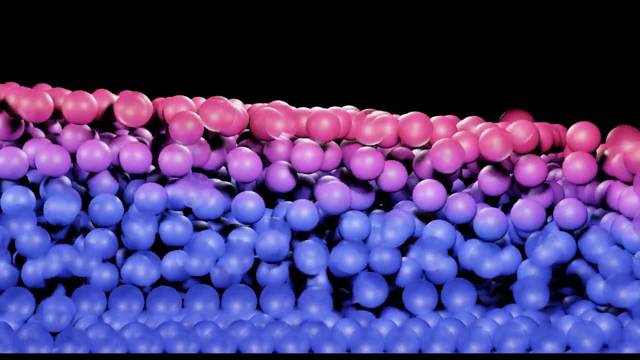 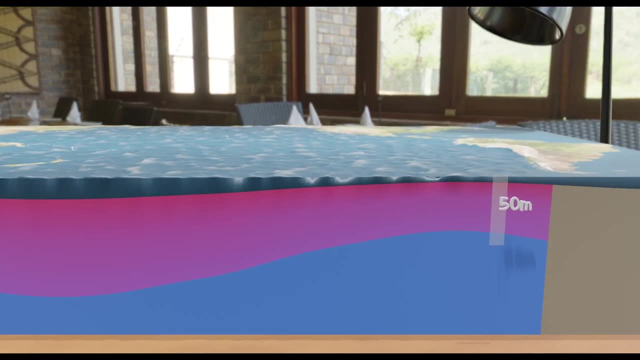 replaced, so water from below rises to do so. Here's where our thermocline comes into play. The thermocline in the east is very shallow, less than 50 meters deep. The surface currents created by the wind affect roughly the top 50 meters of water. 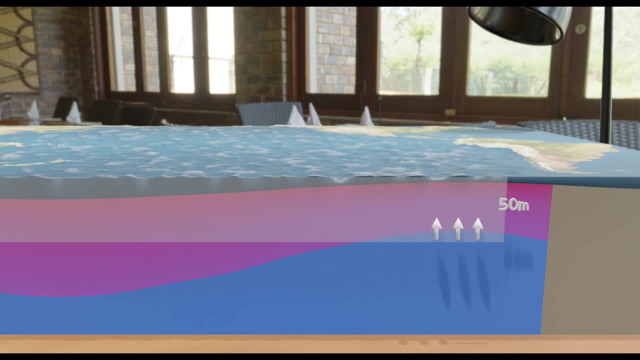 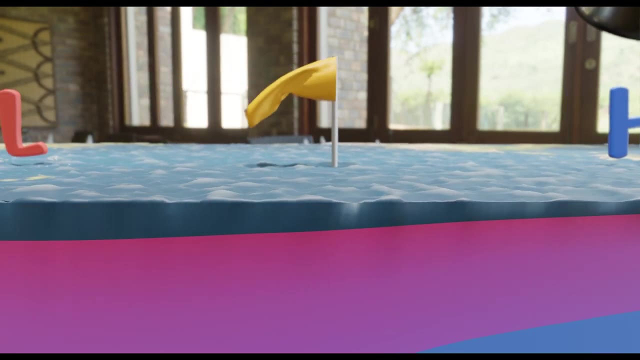 That means the water that rises to replace it comes from below the thermocline, That is to say it's very cold. This keeps our surface temperature cold and keeps our pressure gradient, and subsequently the wind, strong and active, Because the water generally always moves westward and pools up there. the western thermocline. 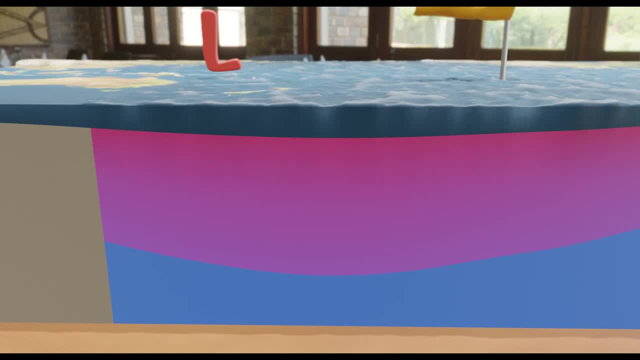 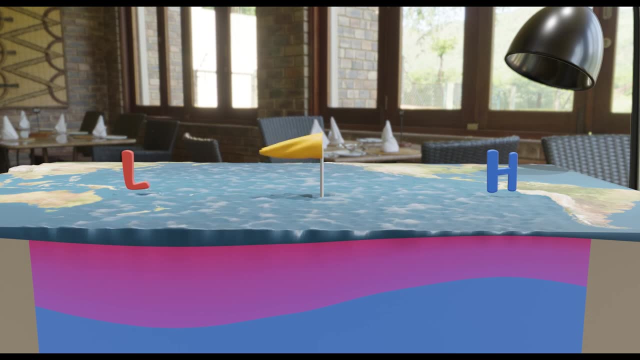 is very deep, causing the surface temperature there to remain warm. So as long as the eastern waters stay cold, things progress normally. El Niño, therefore, is the phenomenon of the eastern Pacific failing to remain cool, But what we have here is a positive feedback loop. 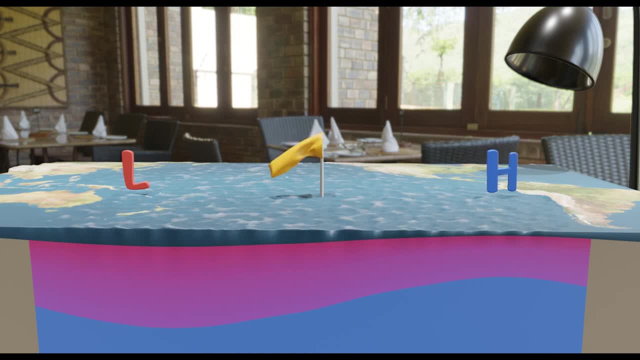 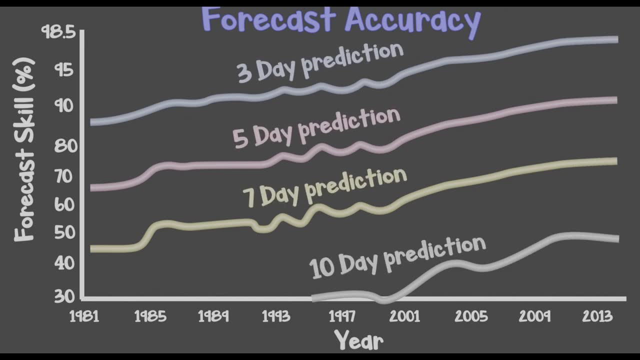 Sure, El Niño is the warming of the eastern, but why does this happen? What breaks this positive feedback loop? What I'm about to present could change in 50 years as computers improve, Because, despite fluids being very simple, calculating and modeling them accurately is. 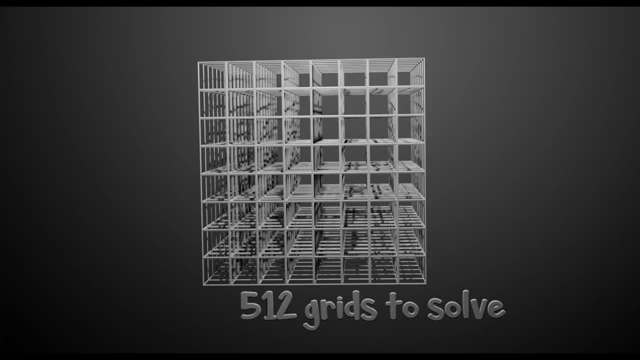 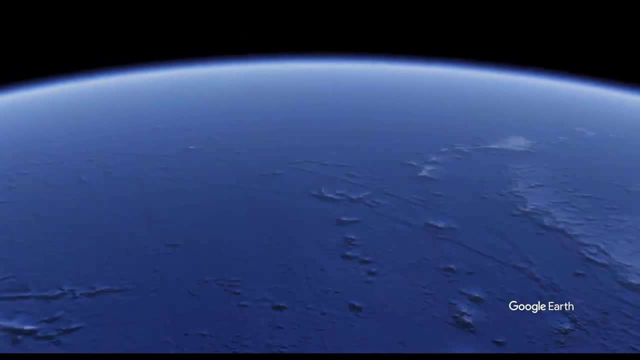 very difficult and it gets exponentially harder as the scale increases. So when talking about the scale of the Pacific, yeah, it's kinda hard to be sure our models are accurate. But what do we think is happening? Earlier I mentioned, there's no reason for the west to be warmer than the east. 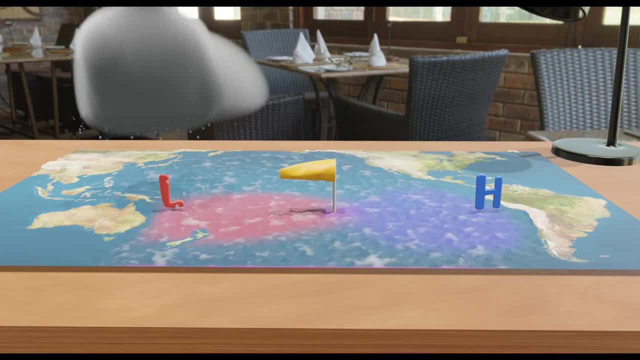 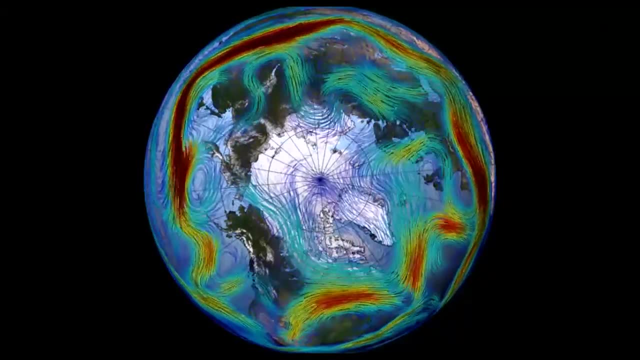 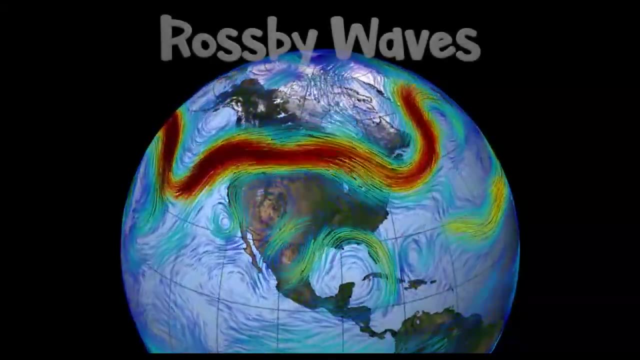 That's right. Both points are along the equator and receive the same amount of light. So how does this imbalance occur? Any fluid on a rotating sphere like earth is affected by the sphere's rotation. This manifests in lateral motions we call Rossby waves. 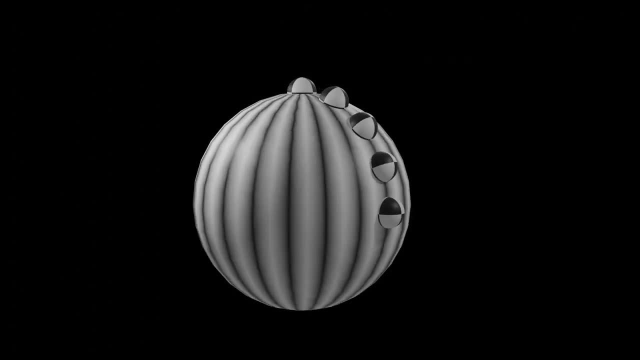 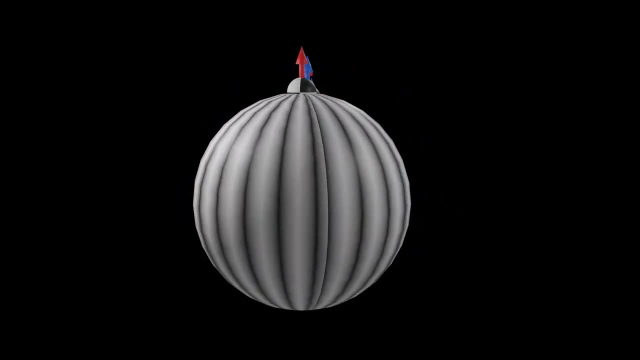 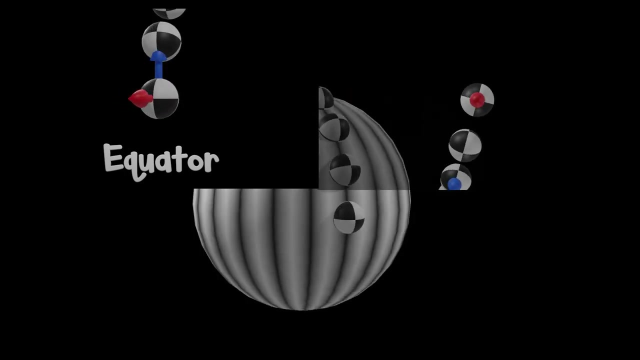 If we imagine a distribution of particles along a single longitude of earth, we can compare their relative rotation in space compared to their rotation along the normal axis. Here, 100% of the rotation is on the y-axis and none along the normal, Whereas in the poles 100% of the rotation is along the normal. 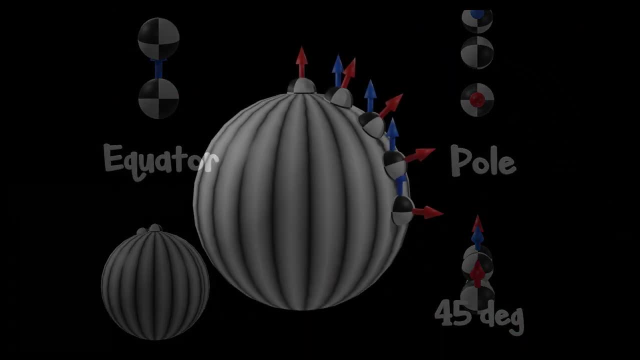 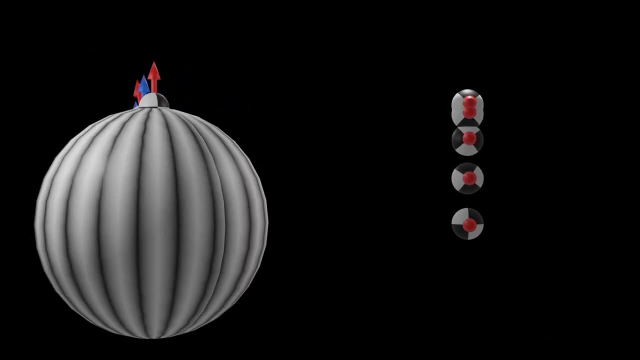 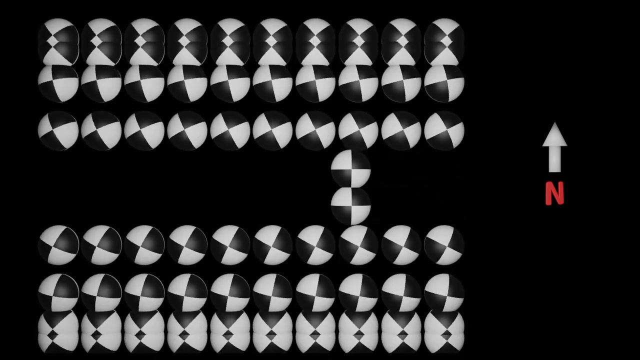 If we compare the relative rotation along the normal axis, we can see that water particles rotate faster as they move away from the equator. What's this mean? Any water that moves slightly away from the equator will encounter faster rotating water particles that will push them to the west. 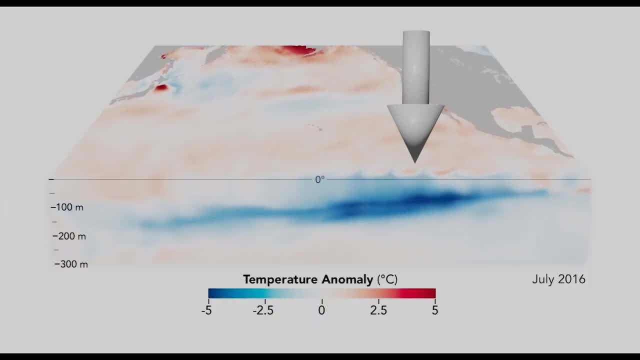 Opposite, As one would expect from the Coriolis force. This push to the west creates our Rossby waves, and thus we get the start of how our Pacific should look. As this water travels west, it starts building up and pushing down the thermocline which 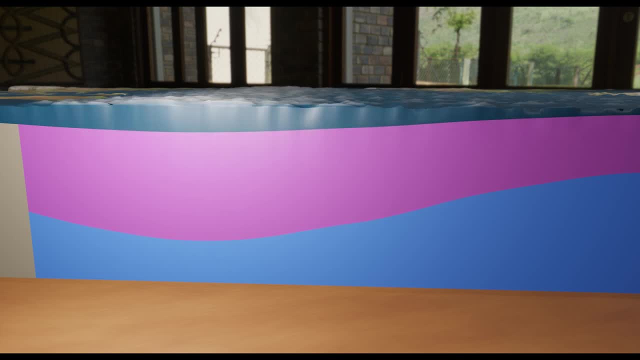 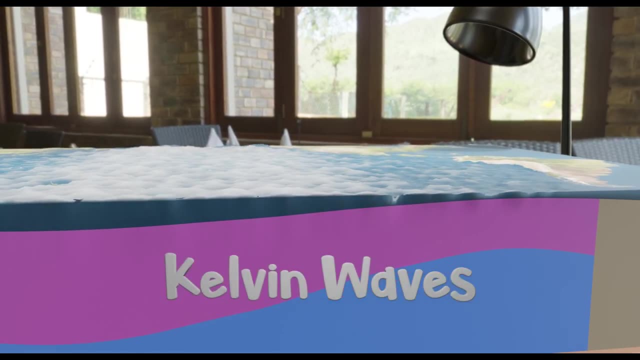 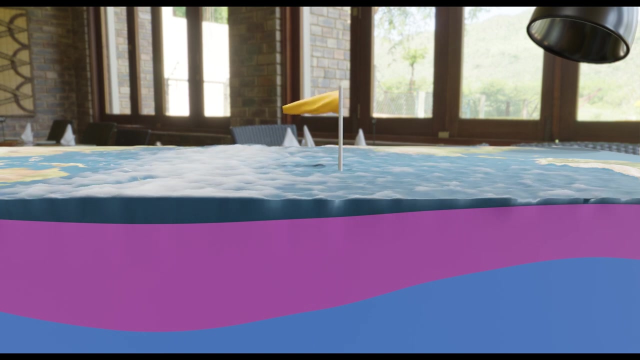 is a criteria needed to keep the western Pacific warm. These arriving Rossby waves also reflect off the western coast and begin their journey back east as what we call a Kelvin wave. But the Kelvin wave is of lesser impact than the Rossby waves Because the Rossby waves are soon reinforced by easterly wind flows. 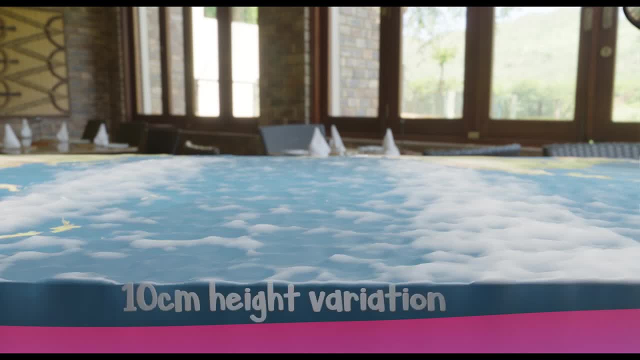 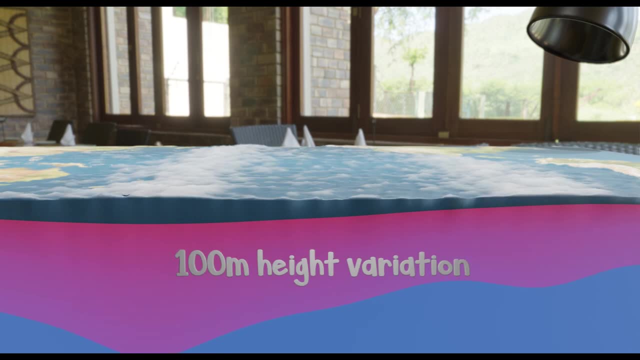 Rossby and Kelvin waves can be detected at the ocean surface, but they are only roughly 10 centimeters in height. However, in the thermocline these waves can cause fluctuations of up to 100 meters- Huge variations in thermocline depth. 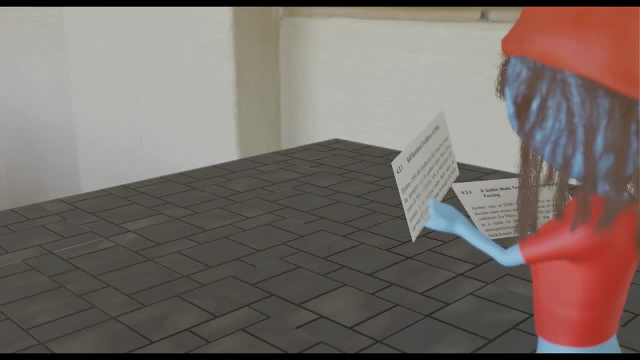 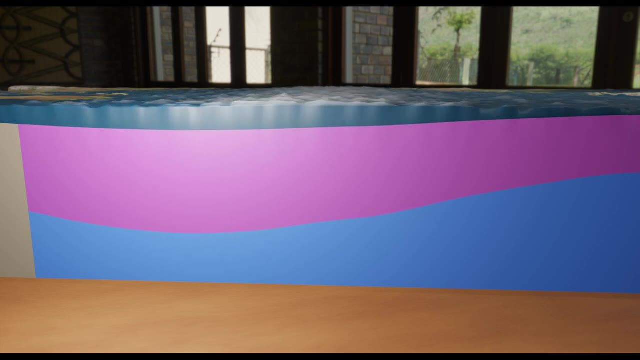 Now we've reached the disputed part of our El Nino. What causes the tipping point? We've seen how Rossby waves can create waves. We've seen how Rossby waves can create waves. We've seen how Rossby waves can create warm water buildup in the west, which pushes 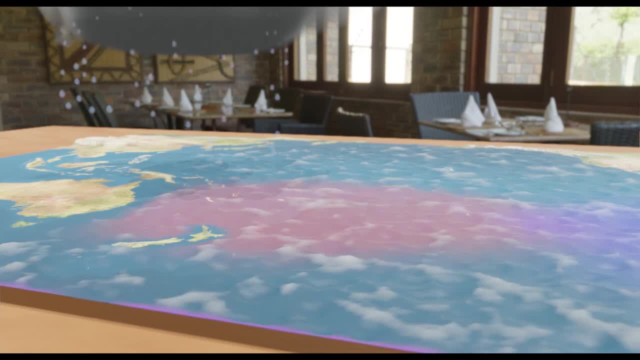 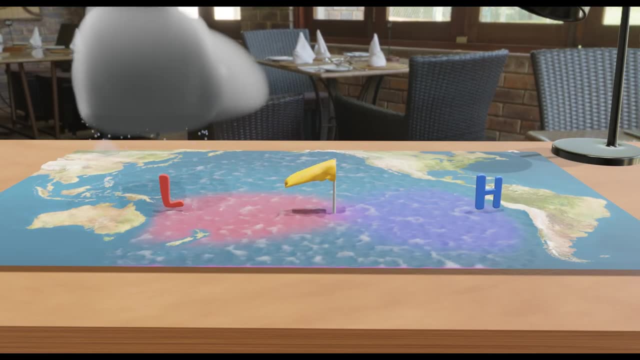 down the thermocline, keeping the water warm. This warmth creates a low pressure region which causes winds to blow from east to west. This wind brings more water and also helps amplify the cool surface water in the east, thus continuing the cycle. So how do we break this positive feedback loop? 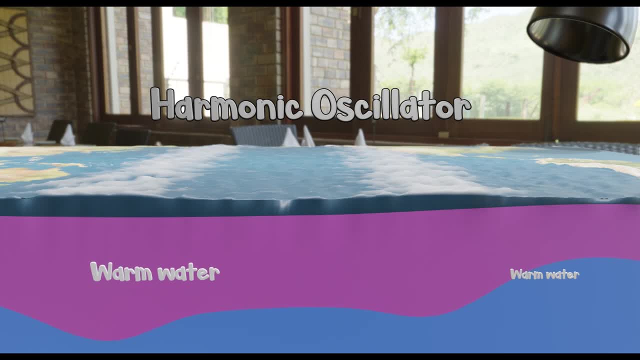 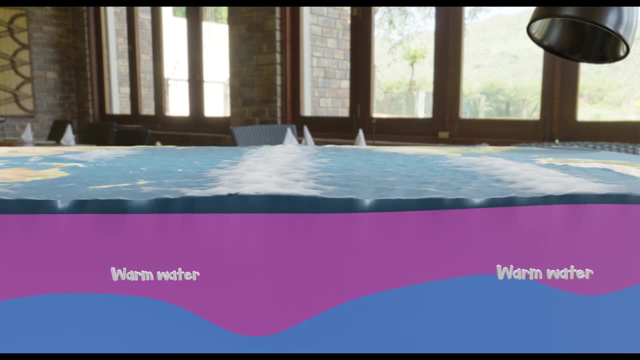 There are two main theories. The first is that there is a natural oscillation between buildup of warm water in the west, followed by reflection of waves to the east. This reflection then pushes down the thermocline as it goes and warms the ocean's surface. 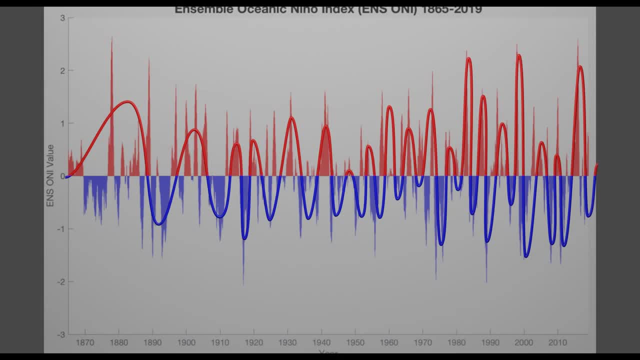 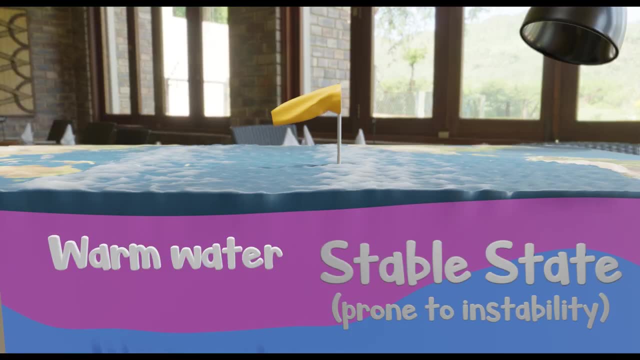 This oscillation can be affected by noise or interactions with the atmosphere. There's also a more stable yet stochastic model, which suggests that this buildup of warm water in the west is a stable state, as long as the winds and currents holding it there are maintained. 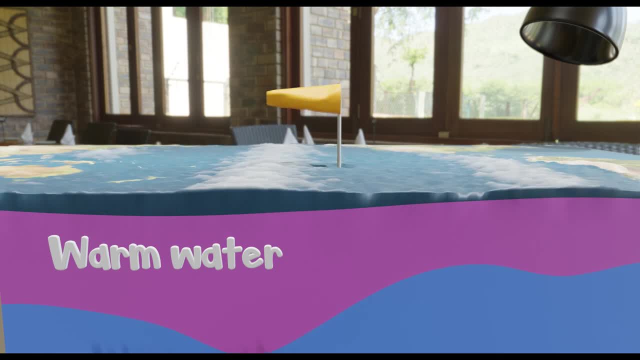 But of course nature isn't constant And eventually there will be some disruption, And eventually there will be some disruption. Second, there's a slip. as I like to visualize it, This slip causes the warm water volume to destabilize and discharge from the western. 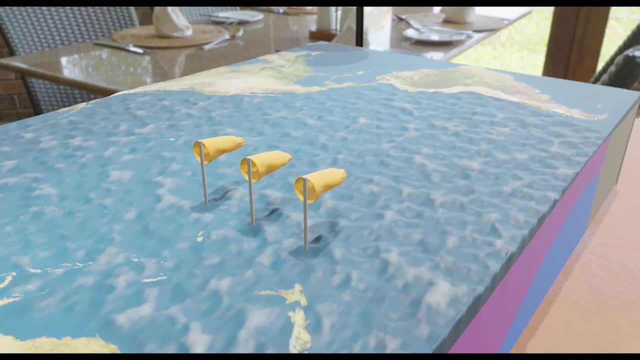 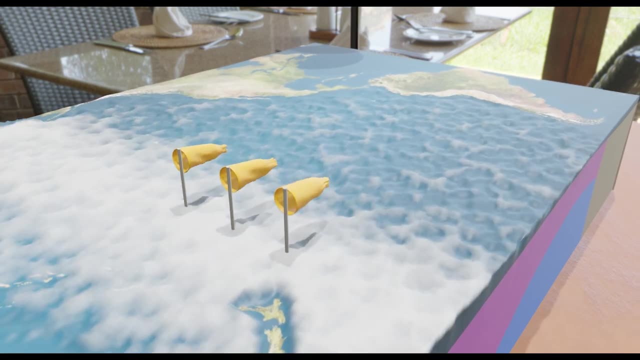 pacific, There is decent correlation between strong westerly wind events and the initiation of Nino events. These strong winds push the warm water east, starting the discharge. The produced kelvin waves then flow to the east, lowering the thermocline as they travel. 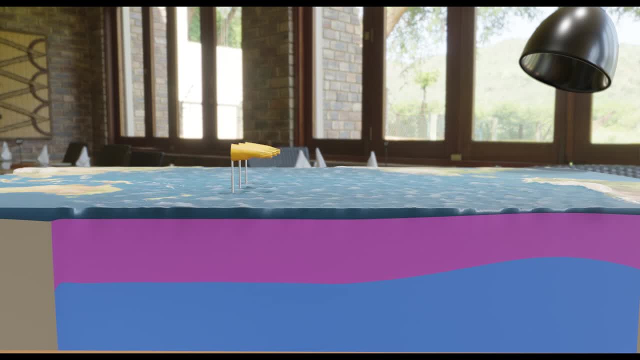 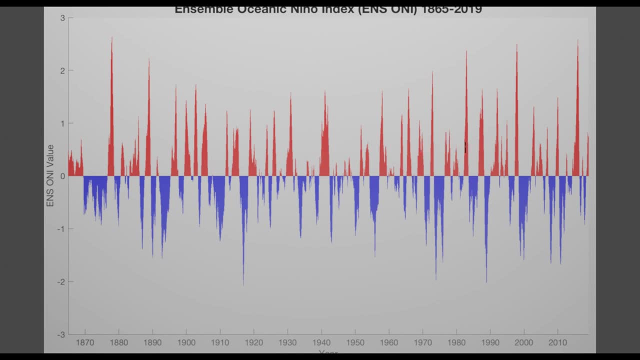 while subsequently raising the thermocline in the west. This model is a bit more attractive as it can explain how or why mini-events have different timings and variabilities and strengths. But both models look rather similar and perhaps they are one and the same. 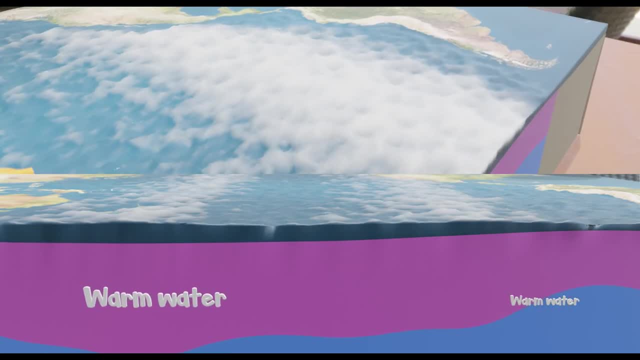 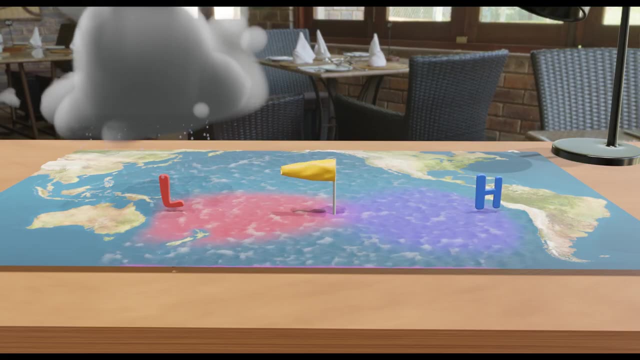 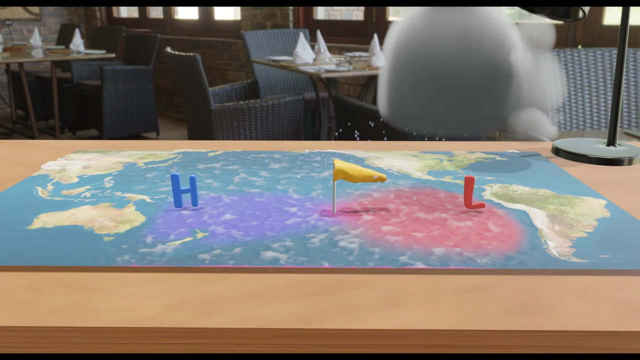 Only stronger computing power may tell us for sure. Because of the redistribution of the warm water and change in equatorial thermocline, we have a reversal in ocean temperatures: Warmer in the east, cooler in the west. And since ocean temperatures affect climate, 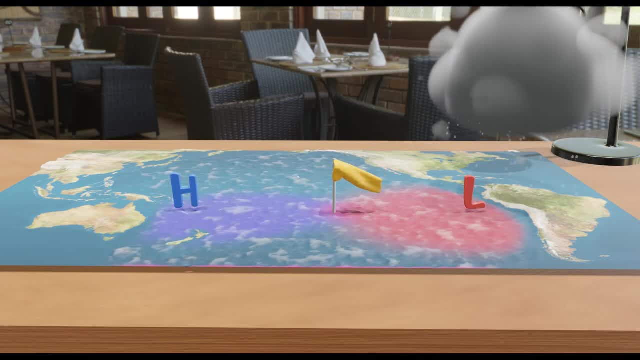 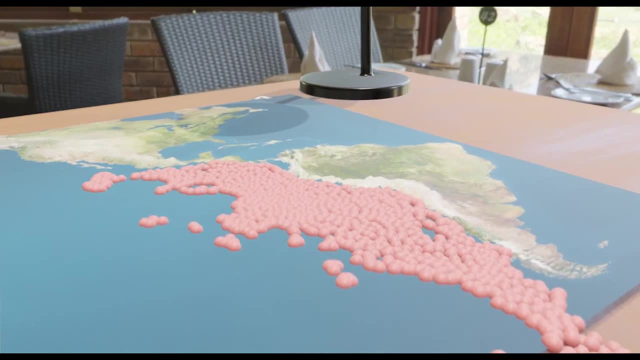 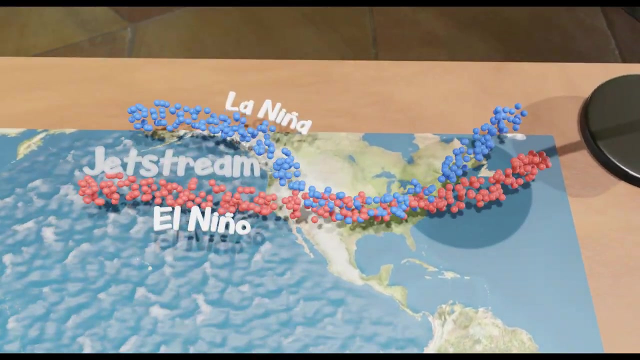 we see drastic changes in the climate in the east and west. As this warm water reaches the east, it collides with the American coasts, dispersing to the north and the south. These changes in temperature affect not only ocean currents, but atmospheric currents too. We aren't quite sure how and to what extent it does. 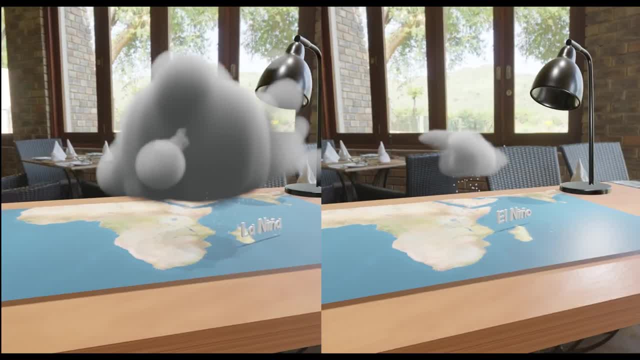 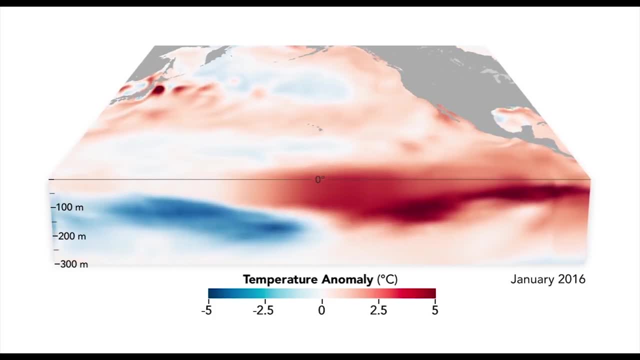 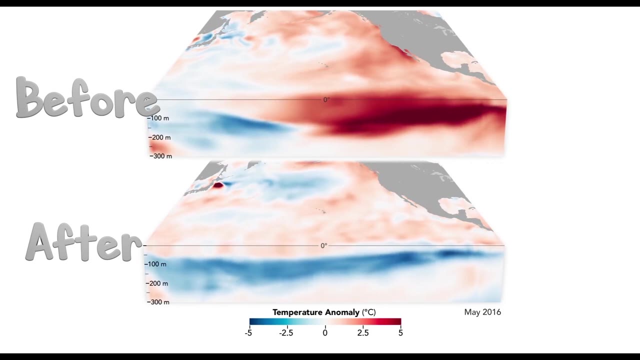 but someday we may be able to explain how exactly El Niño causes climate impacts all over the globe. After an El Niño event, the warm water content in the equatorial Pacific is drained, and thus the process starts over. Lastly, as a quick addendum, I should mention that the scientific community has agreed on the